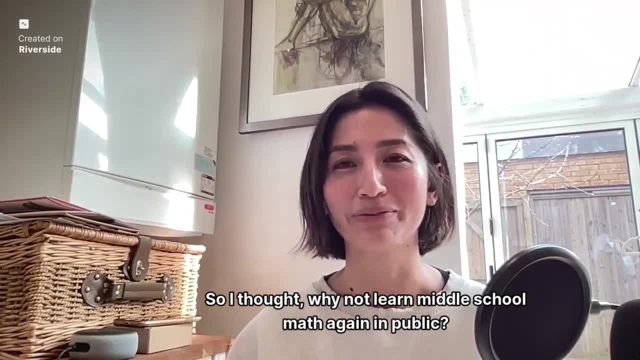 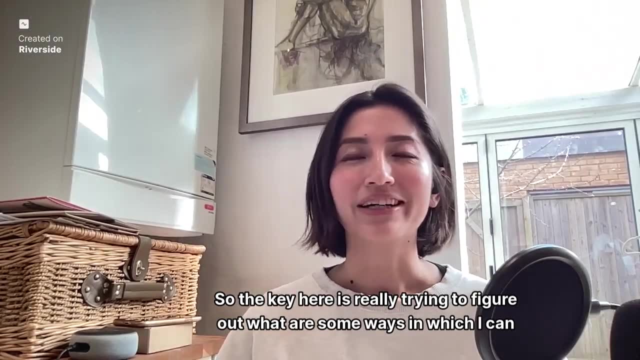 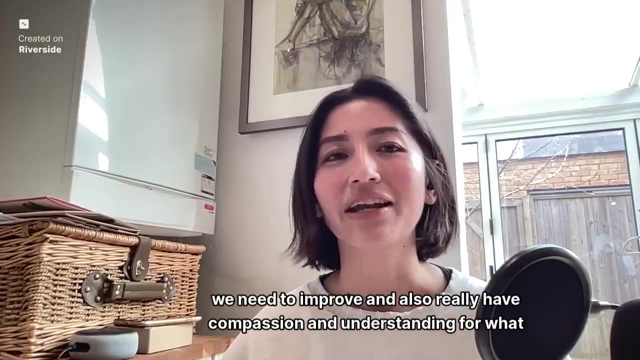 pretty stressed, So I thought, why not learn middle school math again in public? So the key here is really trying to figure out what are some ways in which I can improve this AI teacher so that I can better understand what we need to improve and also really have compassion and understanding for what. 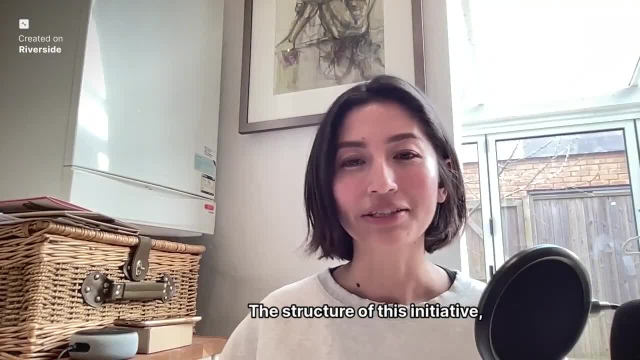 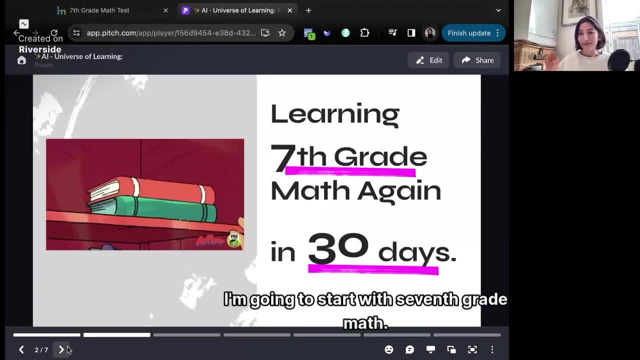 middle school kids are going through and what my cousins are going through. The structure of this initiative is learning math with my AI co teacher. I'm going to start with seventh grade math. I'm going to do it in 30 days. Hopefully I stick with it. now that I'm uploading the videos, I think I probably will need to do that. 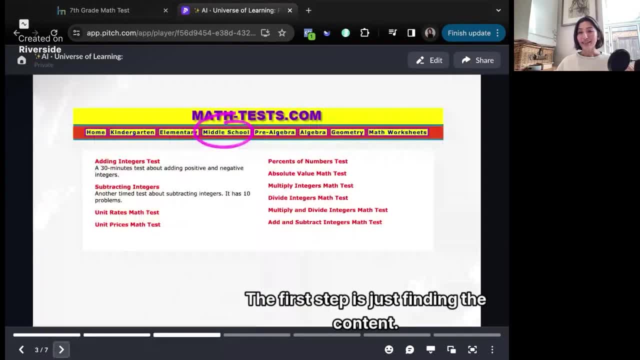 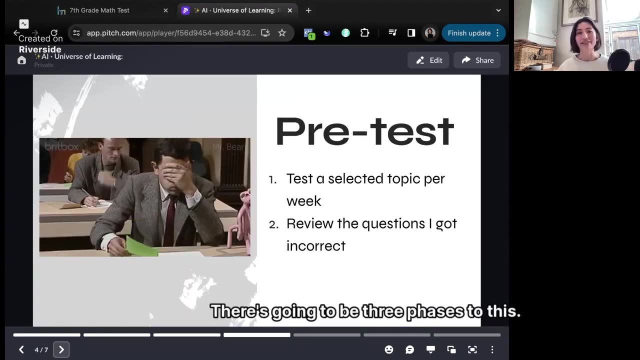 just for accountability myself. The first step is just finding the content. So there's this website called mathtestcom. I found a seventh grade math section and there's a bunch of topics on here that I'm going to go through on a weekly basis. There's going to be three phases to this. The first phase is the. 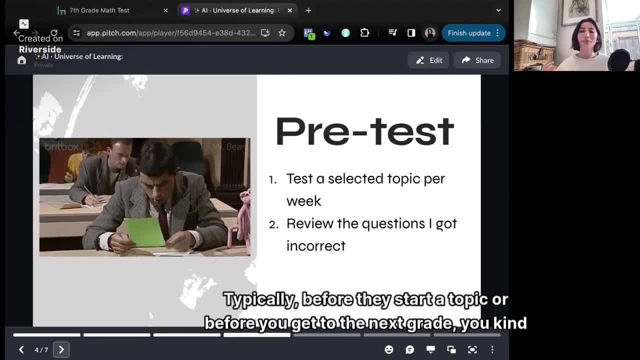 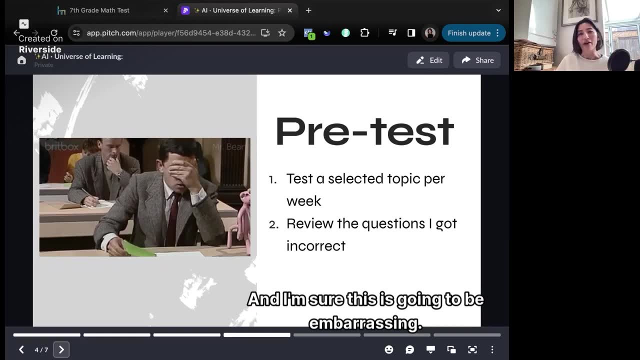 pre-test, And this is what they do in schools Typically, before they start a topic or before you get to the next grade, you kind of do a pre-test to see where you are, And I'm sure this is going to be embarrassing. I'm going to select a topic per week. I'll do the test and review the. 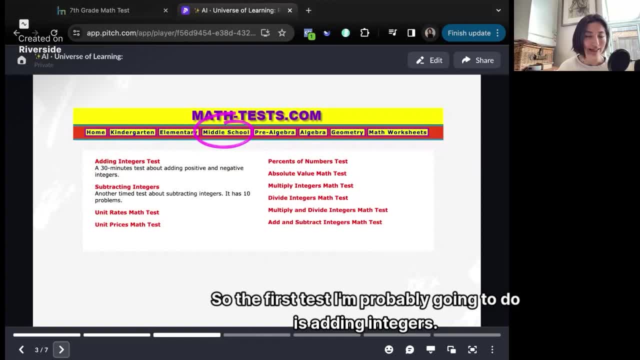 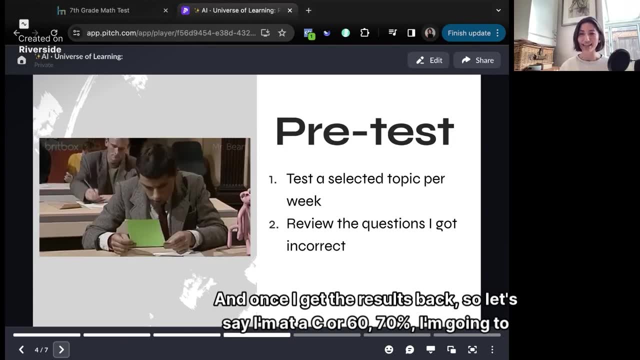 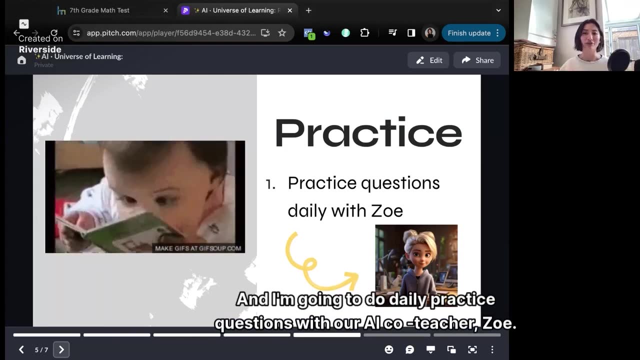 questions that I got incorrect. So the first test I'm probably going to do is adding integers And once I get the results back- so let's say I'm at a C or 60, 70%- I'm going to review the questions that I got incorrect And I'm going to do daily practice questions with our AI co-teacher. 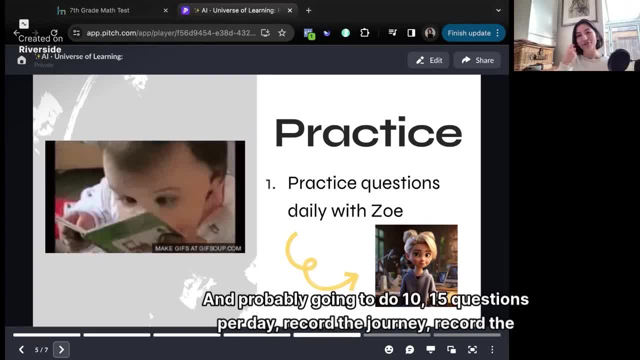 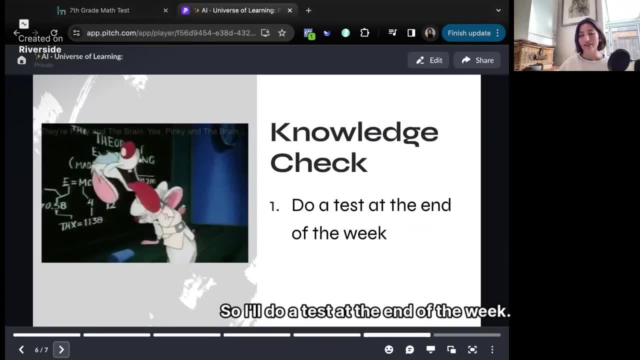 Zoe And probably going to do 10, 15 questions per day, record the journey, record the practice And then at the end of the week I'm going to do a knowledge check. So I'll do a test at the end of the week and compare my score Zoe can generate. 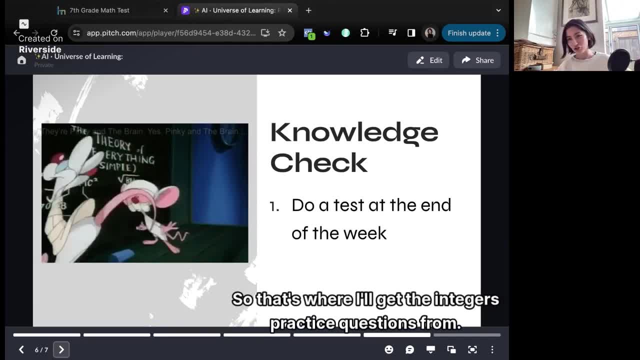 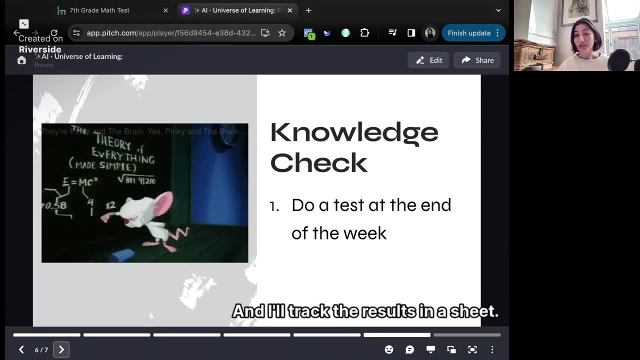 practice questions for me. So that's where I'll get the integers practice questions from, And I'll also ask her to help generate a 10 question test that is similar, if not maybe even slightly harder than the initial test that I did, And I'll track the results in a sheet And hopefully by the 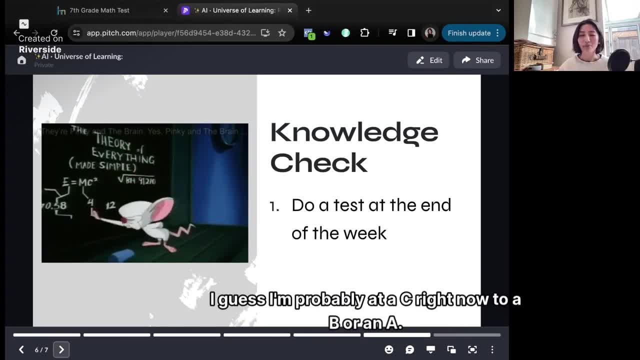 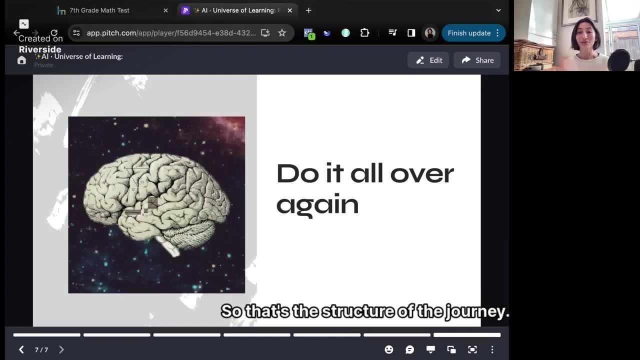 end of the 30 days I've moved up from- I guess I'm probably at a C right now- to a B or an A, And then I'll do it all over again each week. So that's the structure of the journey. 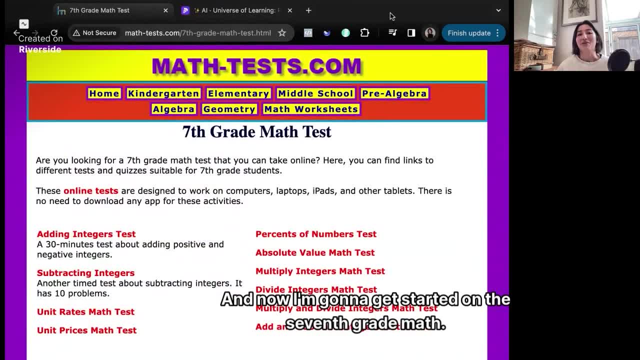 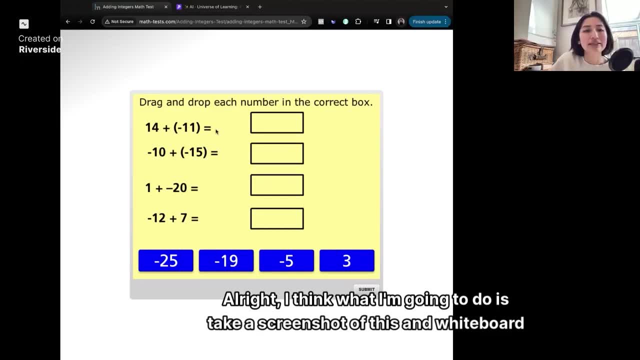 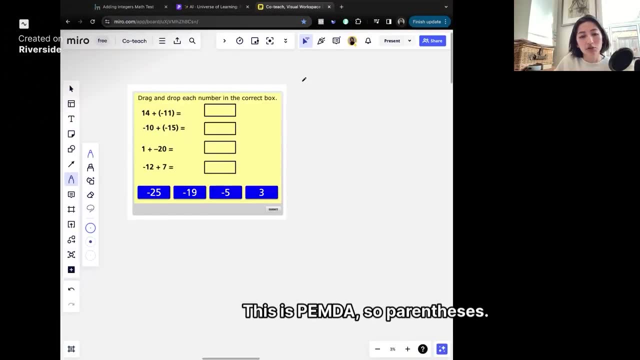 And now I'm going to get started on the seventh grade math test. I feel like that's probably it. All right, I think what I'm going to do is take a screenshot of this and whiteboard it. Okay, This is PEMDA, So. 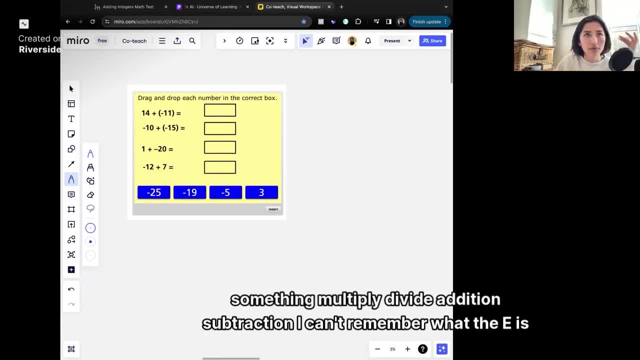 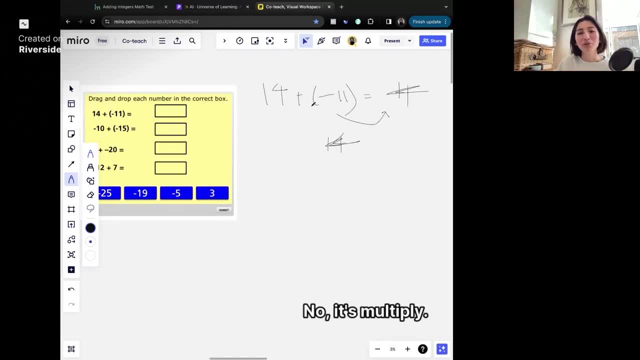 parentheses something: multiply, divide, addition, subtraction. I can't remember what the E is. Okay, So, oh no, no, it's multiply. Okay, So 14 times negative 11. This is so hard Because I feel like that would be like negative in the negative hundreds. So that's probably not. 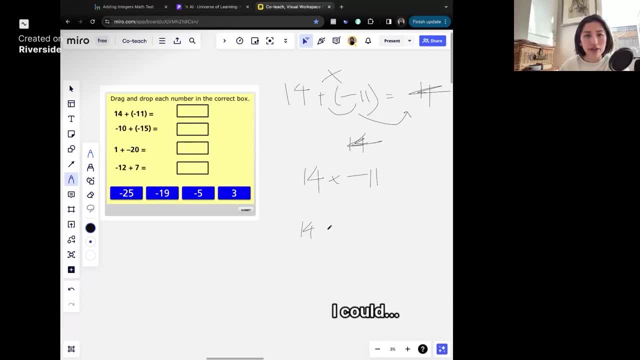 right. Oh man, I feel like I could. let's try this again: PEMDA. So it's parentheses, parentheses. first, I have to take out the parentheses. Oh, okay, Now I got it, because positive and a negative multiplied is a negative. 14 minus 11 equals three. Yes, Okay, Here we go. 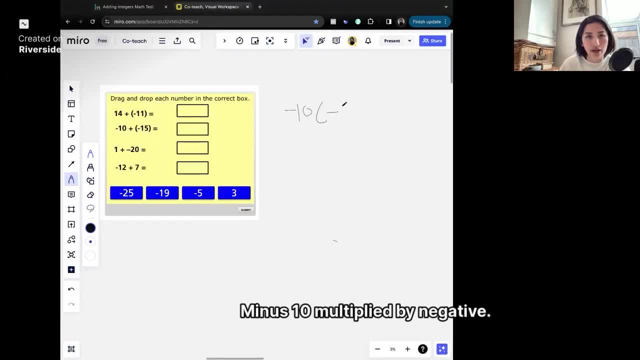 All right, Minus 10 multiplied by negative. Do the same thing. So multiply these, then you get minus. So that's minus 10.. Oh yeah, I'm getting it Minus 15.. So that's negative 25.. Okay, Okay. 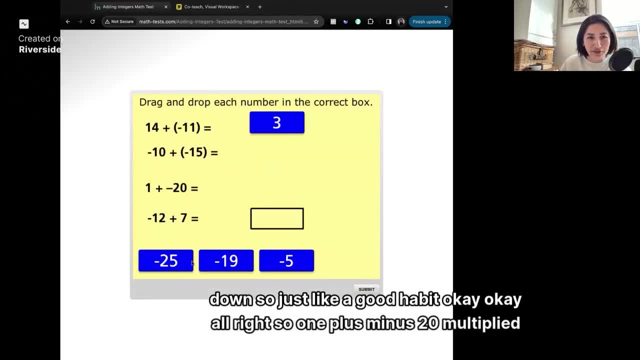 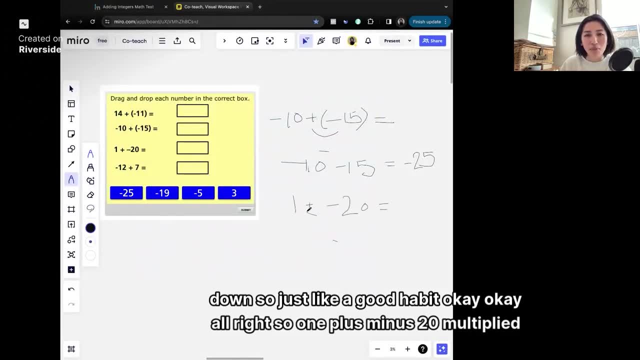 I should probably write that down, So just like a good habit. Okay, All right. So one plus minus 20 multiplied. No, not multiply, because that's not in parentheses, So I will: one equals. no, maybe that is okay. One plus my. 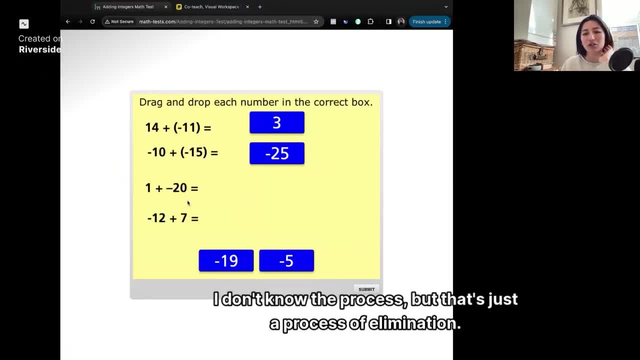 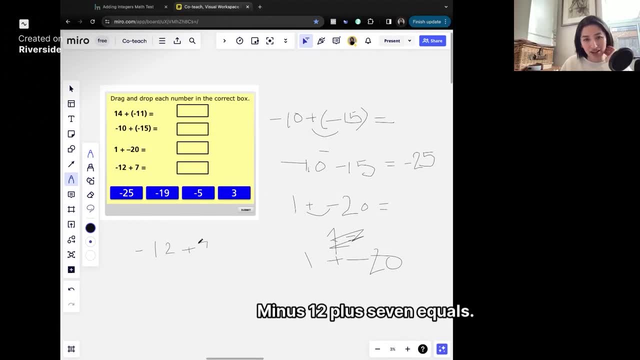 I just feel like it would be negative. 19, because it's 20 and one. I don't know the process, but that's just a process of elimination. 12 plus seven equals. No, that's not Okay. I'm just going to whatever. I'm just going to do. 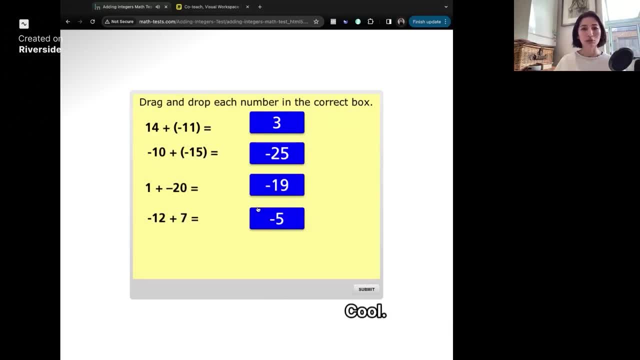 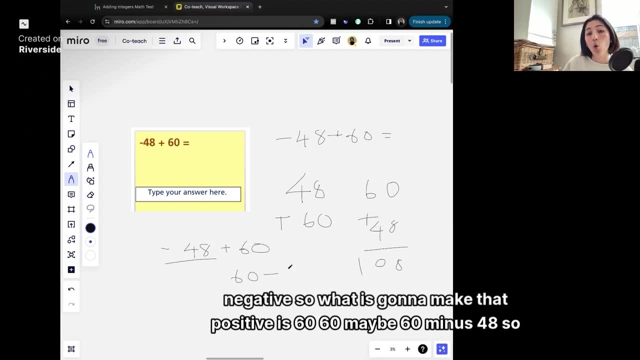 this: Oh, okay, Cool Cause it's negative. So what is going to make that positive is 60.. Oh, 60, maybe it's 60 minus 48.. So that's five, That's 10 too, Okay, I feel like. 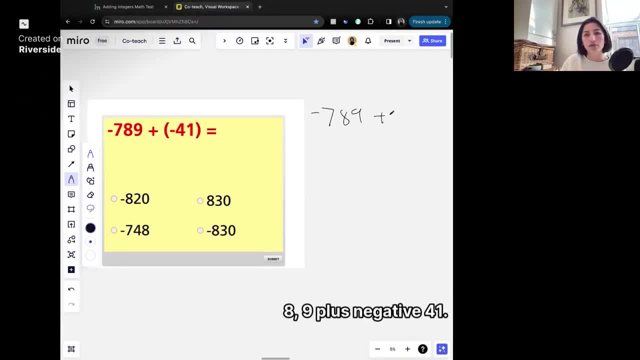 I've got it Okay. Nine plus negative 41. So we multiply, So that's negative, So nine is negative. seven, eight, nine minus 41. Okay, So that's 10,, 12,, 13,, eight, So that would be. 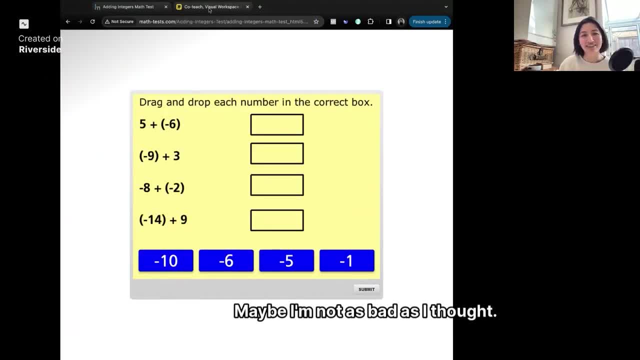 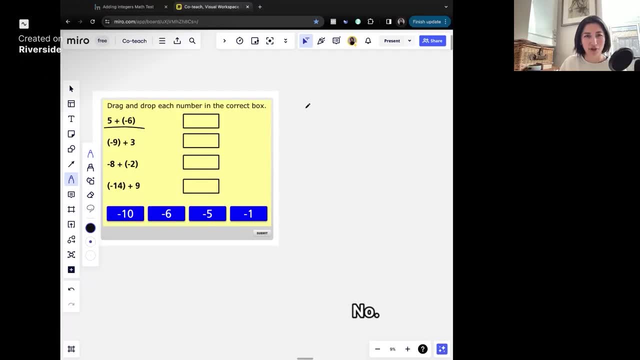 negative. Maybe I'm not as bad as I thought. All right, let's do this. So this is five times six. No, no, that's wrong, Plus three, Maybe that's it. I just I feel like with the 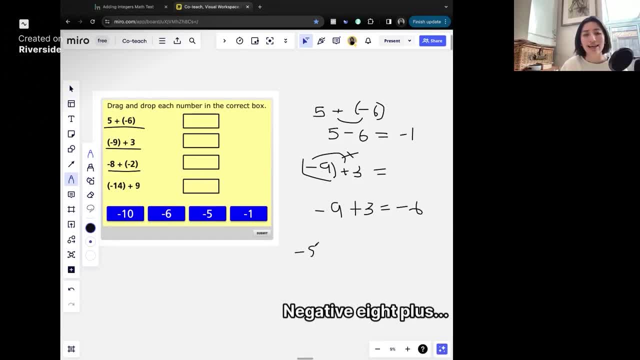 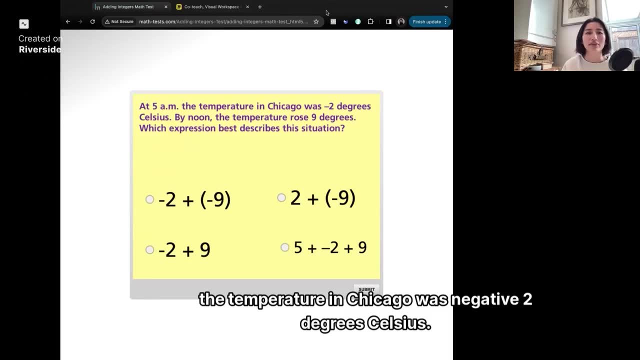 with the minus six. that's probably it, Okay. Negative eight plus. at 5.00 AM The temperature in Chicago was negative two degrees Celsius. by noon The temperature rose nine degrees, which expression best describes the situation? The temperature rose So that. 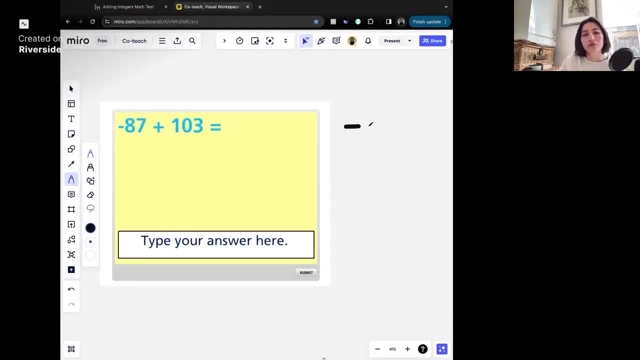 is probably okay, People. what's 17 minus nine? So I think that's just going to be one. Oh, three minus 87.. That's very weird. Um, okay, I'm just going to try. I just don't think that that's. 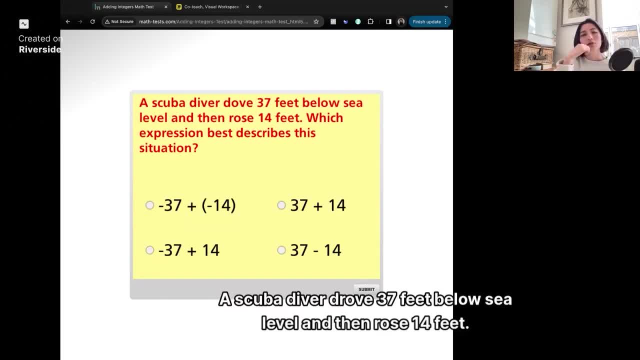 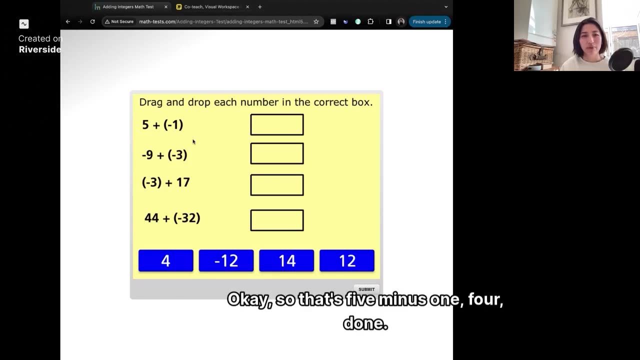 right, Uh, a scuba diver drove 37 feet below sea level and then rose 14 feet. which expression best describes this situation? I didn't think it was bad enough, Okay, Okay. So that's five minus one. four Done Negative. nine minus three, That's nine plus three. 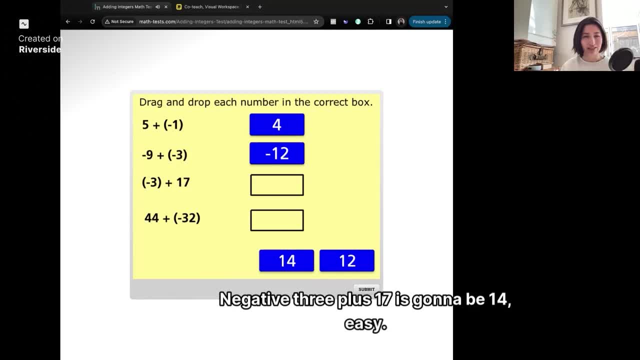 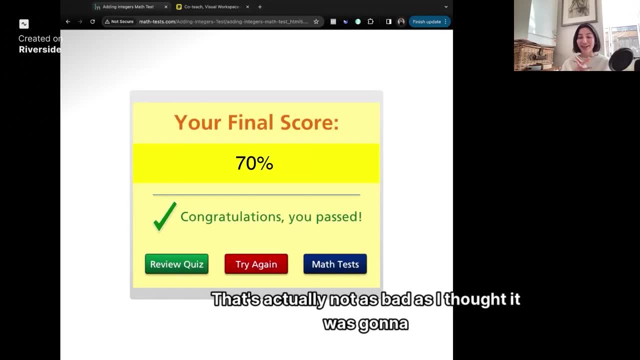 is 12.. Negative: 12.. Negative: three plus 17 is going to be 14.. Easy, 44 minus 32.. That's 12.. Okay, cool, Great. That's actually not as bad as I thought it was going to be. So I've done the. 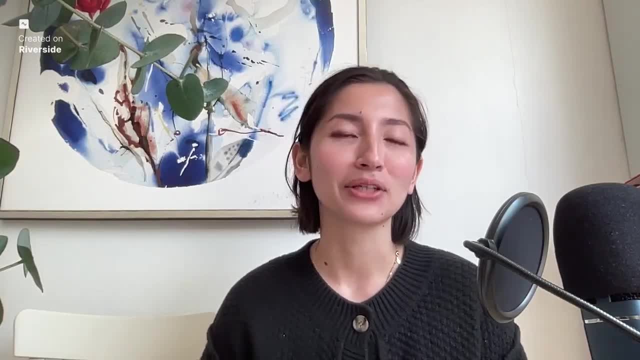 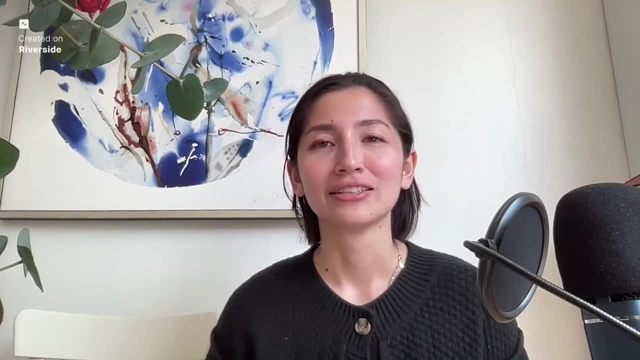 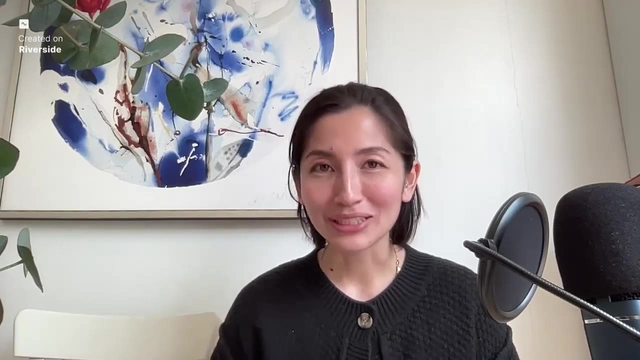 first seventh grade math test and now I'm going to practice the questions I got wrong And I'll do five practice questions per question I got wrong, So that'll be 20 questions this session and I'm going to do them with Zoe. So I'm going to ask for my co-teachers help to explain how to. 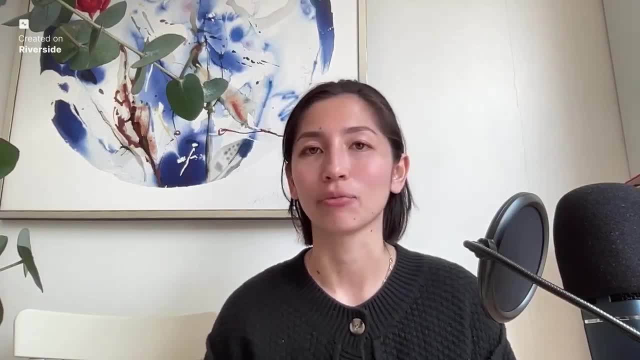 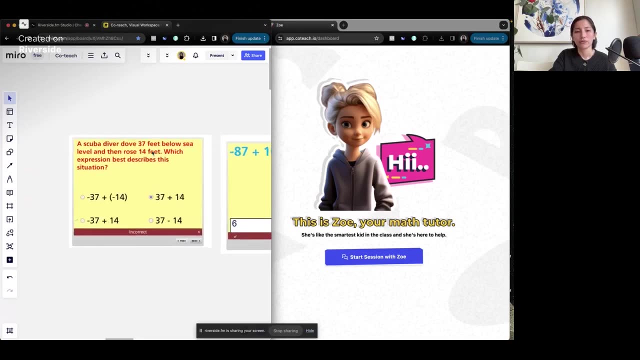 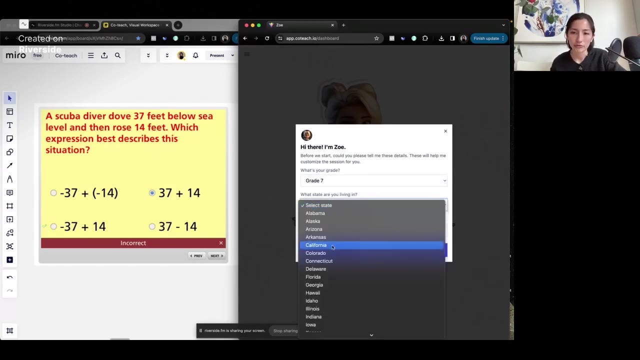 do the question, give me some practice questions and just kind of work through it with her. So let's do this. All right, let's go. So this is the first question I got wrong, So let's start. Seventh grade, California. Oh, I quite like cooking, learning and going on long walks. 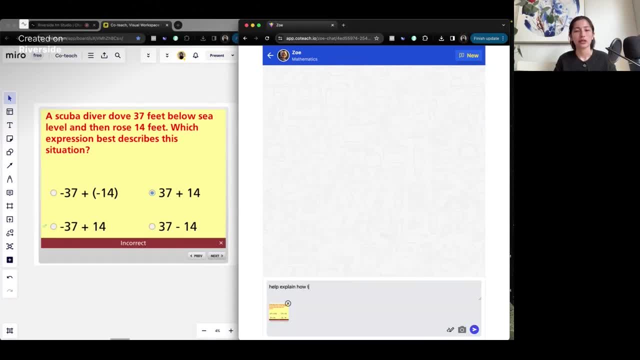 Okay, Help explain how to break down this problem. Oh, let's just try from the top. Okay, When the diver goes below sea level, should we use a positive or negative number? Negative, You know. it'd be really nice, actually, for Zoe to tell me what the question is asking. 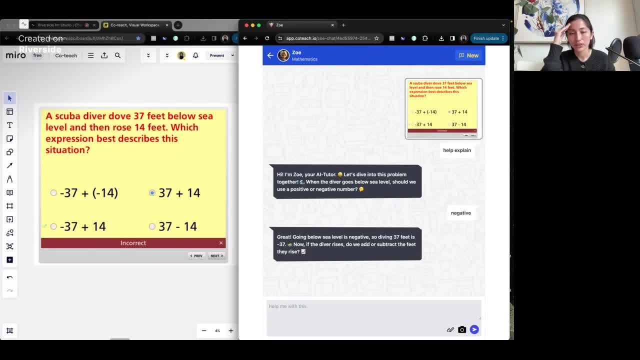 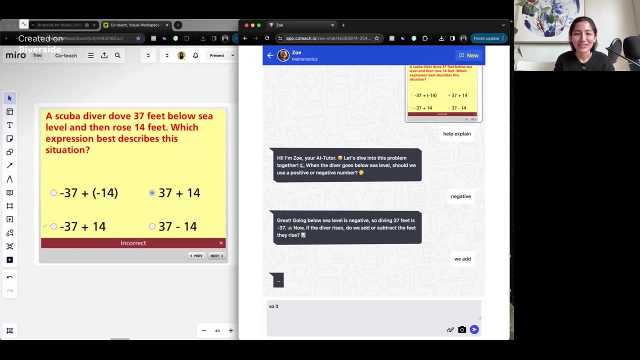 Going below sea level is negative. So diving 37 feet is negative 37.. Okay, Now, if the diver rises, do we add or subtract the feet? they rise, We add, Oh, so it's negative. So it's negative 37 plus 14.. 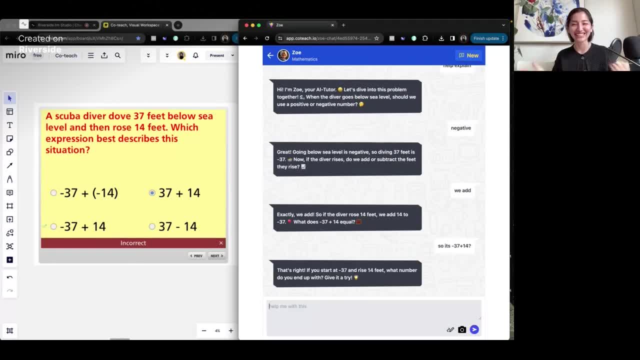 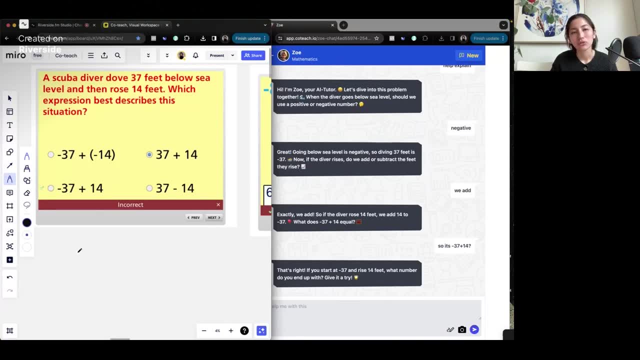 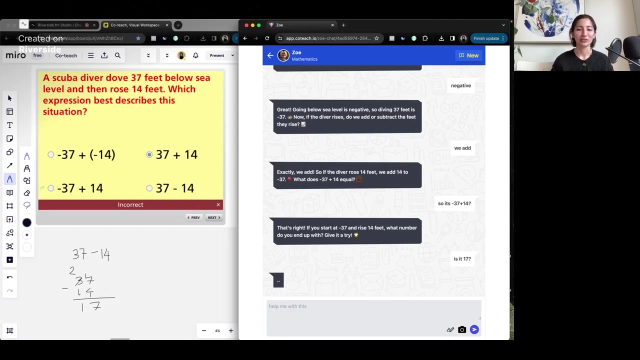 Oh, that's so cool. I actually understood that All right, So I'm going to give that a try. So to do that, I would basically just do 37 minus 14.. Seven one, Is it 17?? Well, actually I could just check with a calculator. Is that wrong? Oh my God, it's wrong. 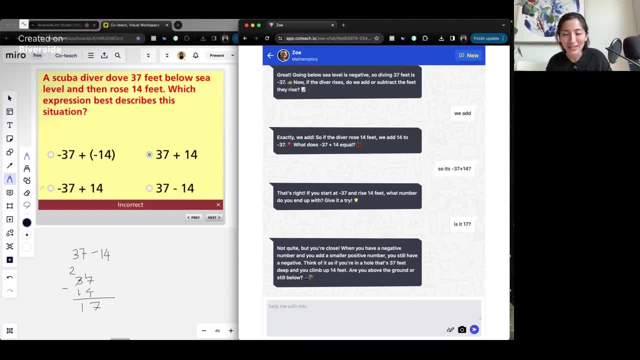 Not quite, but you're close. When you have a negative number and you add a small positive number, okay, you still have a negative. Oh, think of it as if you're in a hole that's 37 feet deep and you climb up 14 feet. 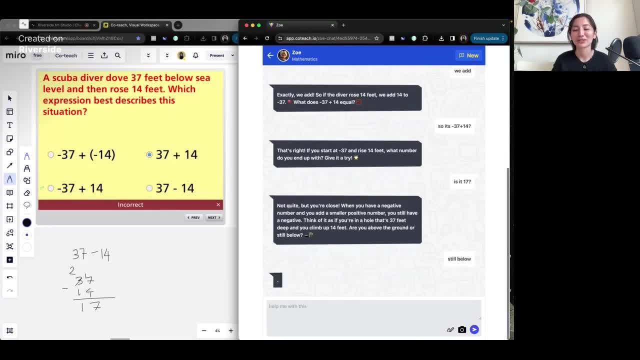 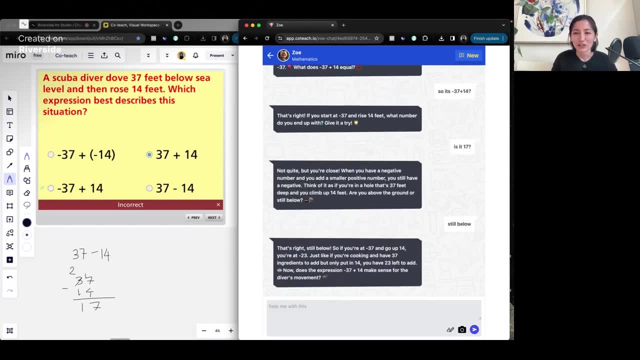 You're above the ground or still below? You're still below, Okay, So of course it's not 17.. It's got to be, Is it? It's got to be negative, Okay. So how do I? so? you're at negative 37 and you go up 14,, you're at negative 23.. 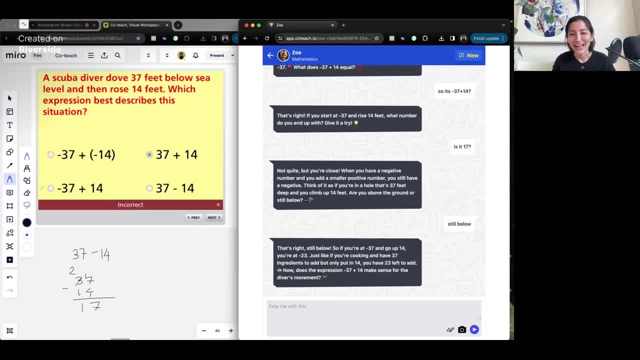 Just like if you're cooking and have 37 ingredients to add, but only put in 14,, you have 23 left to add. Now does the expression negative 37,? can you tell me how to actually do negative 37 plus 14?? 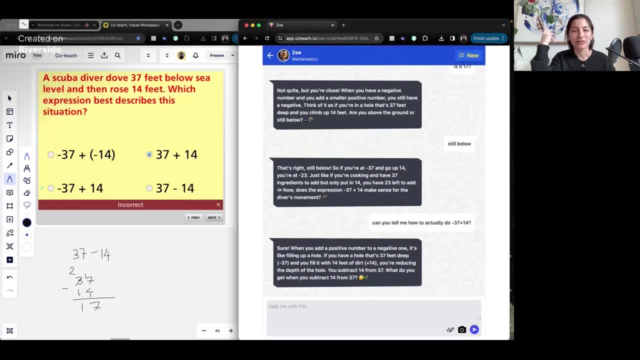 Okay, Now the real test is for Zoe to give me similar- like three or five more similar- questions And to me try to get those right. When you add a positive number to a negative one, it's like filling up a hole. 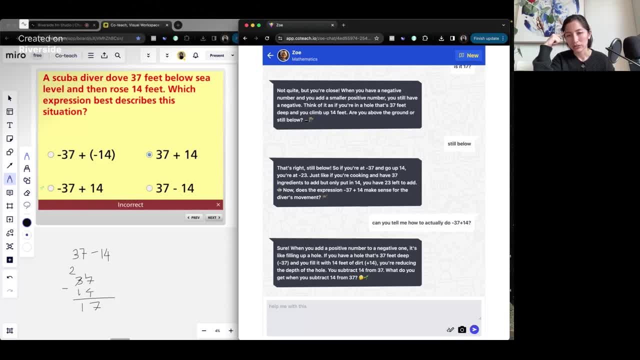 If you have a hole that's 37 feet deep and you fill it with 14 feet of dirt, you're reducing the depth of the hole. You subtract 14 from 37.. What do you get when you subtract 14 from 37?? 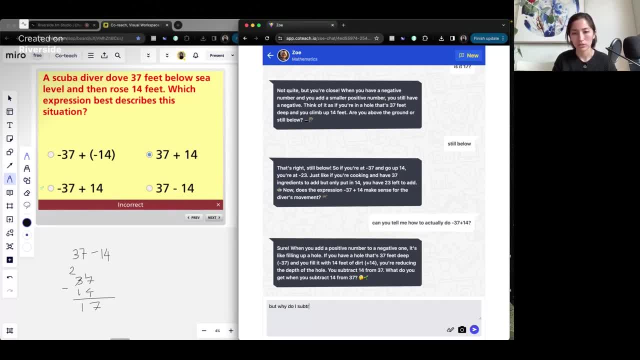 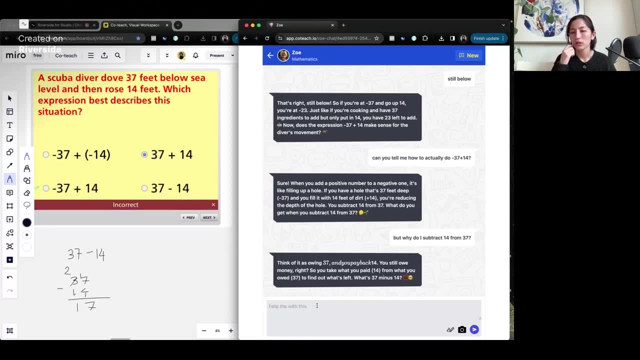 But why? why do I subtract, Think of it as owing 37 and you pay back 14.. You still owe money, right? Yeah, that's true. So you take what you paid 14 from what you owe to find out what's left. 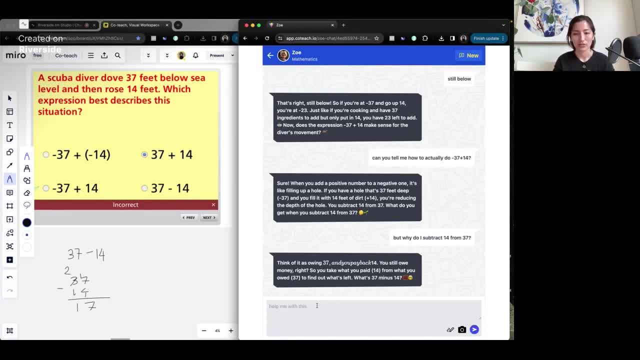 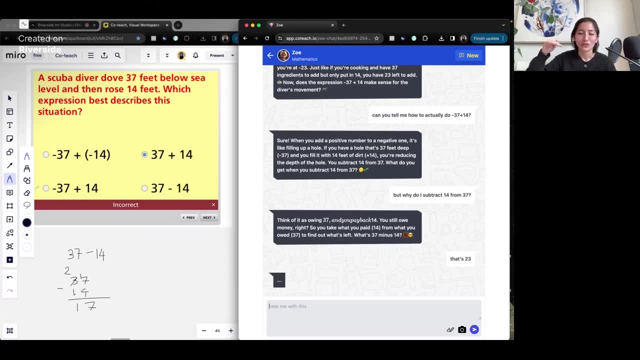 37 minus 14 is 23.. Okay, Gotcha. So I was just minusing my numbers on Okay And then we're still in the hole, So then that's negative 23.. Okay, That is an issue. Why is it italicized like that? 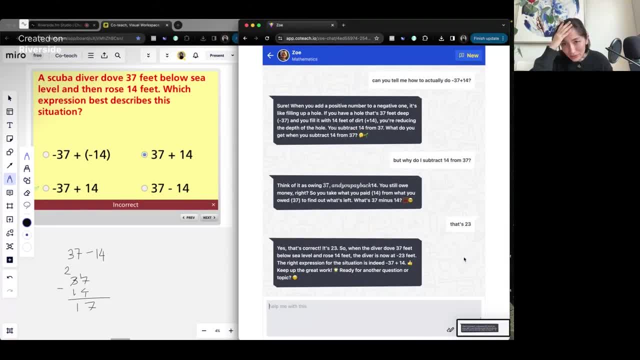 I need to file that. You need to file that bug. Yes, that's correct, It's 23.. So when the diver drove 37 feet and below sea level and rose 14 feet, the diver is now at negative 23 feet. 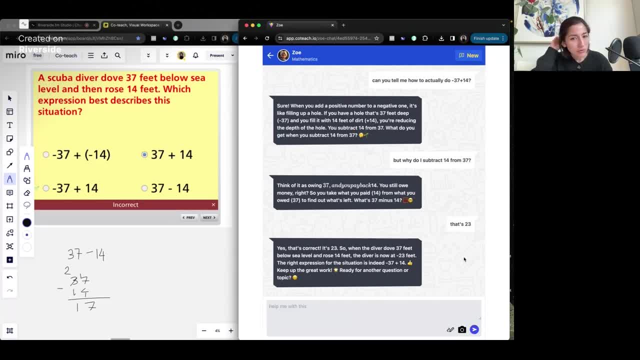 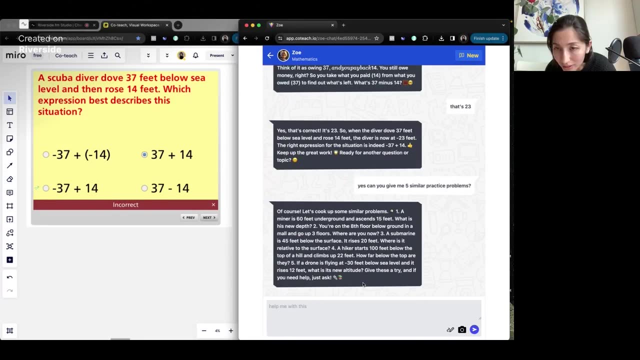 The right expression for the situation is indeed negative: 37 plus 14.. Yes, Can you give me five similar practice problems? That's so embarrassing. Oh, that is super hard to read. A minor is 16.. He's 60 feet underground and ascends 15 feet. 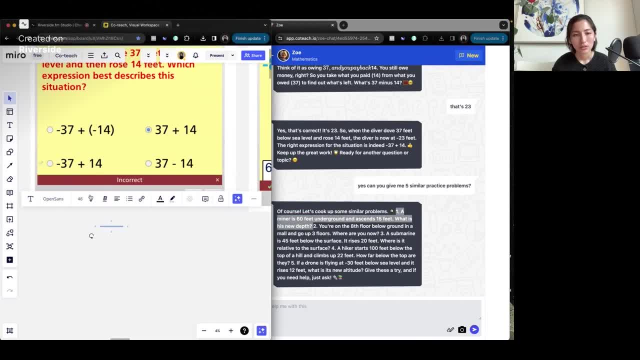 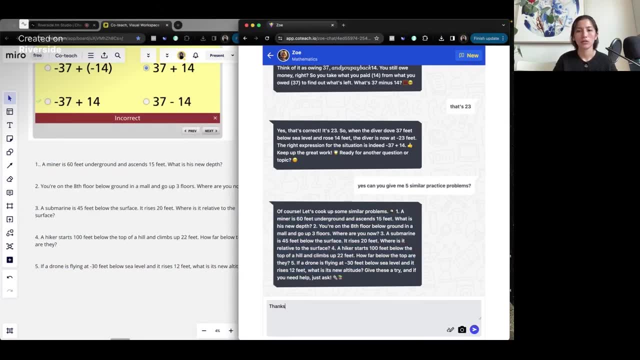 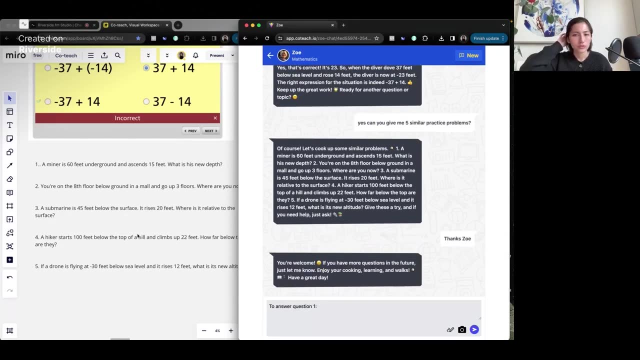 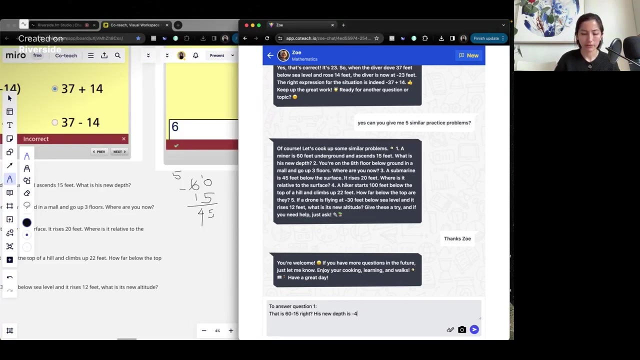 What is his new depth? I'm just going to do this To answer question one. a minor is 60 feet underground and ascends 15 feet, So that's 60 minus 15.. His new depth is negative 45.. Is that correct? 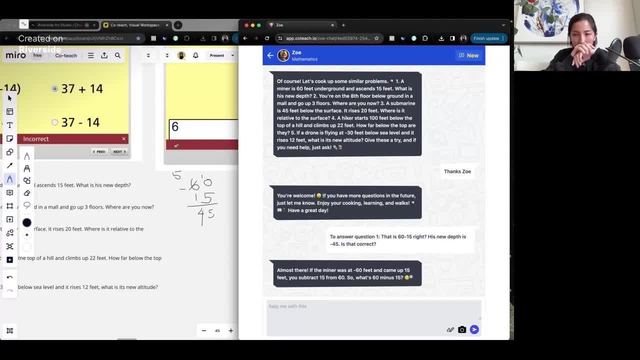 If the minor was at negative 60 feet and came up 15 feet, you subtract 15 from 60. So what is 60?? Well, that's what I said, It's 45. That is really annoying. Okay, Well, I got it right. 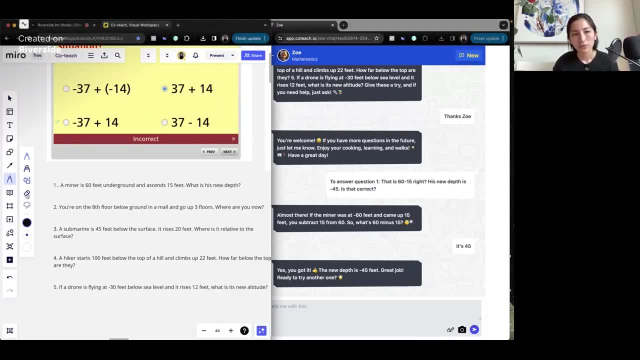 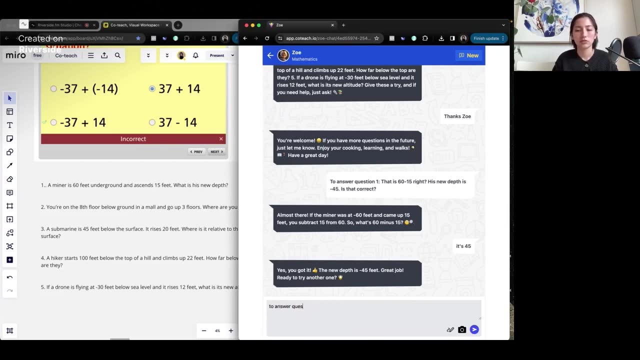 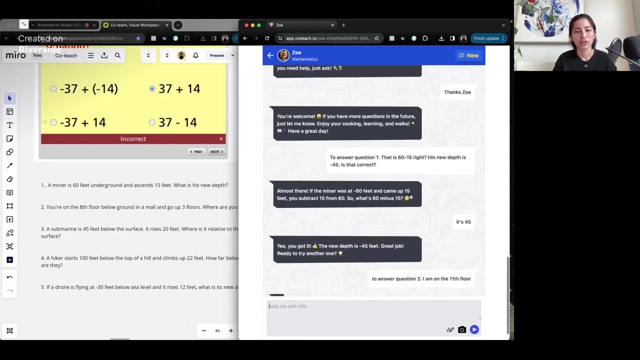 Well, that's something I have to improve. Question two: You're on the eighth floor below ground in a mall and go up three floors. Where are you now? To answer question two, I am on the 11th floor, Oh, below ground. 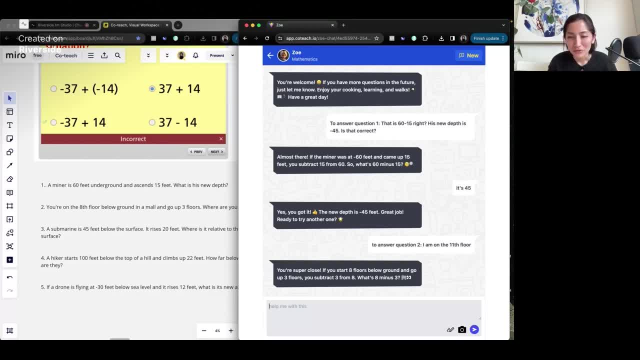 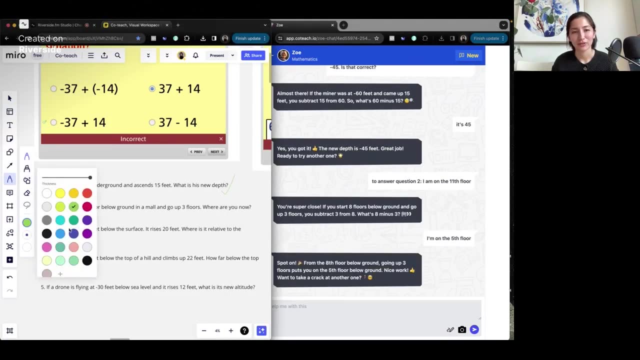 I didn't read that properly. If you start eight floors below ground and go up three floors, then I'm on the fifth floor. Okay, so I got the first. I got this correct. I got this wrong. A submarine is 45 feet below the surface. 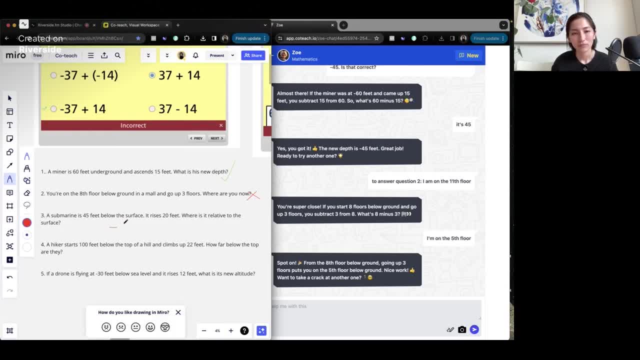 Okay, so that's negative 45. It rises 20 feet, So that's plus 20.. Where is it relative to the surface? So it's going to be to answer question three: negative 45 plus 20 equals negative 25.. 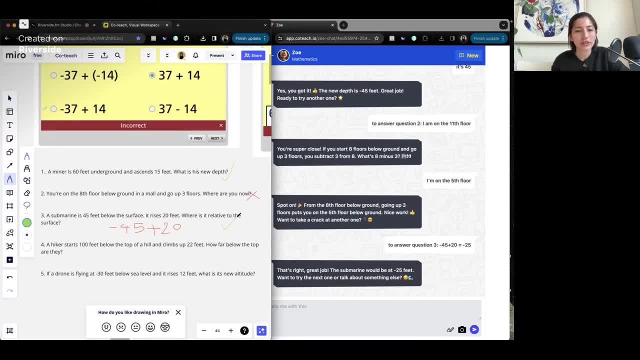 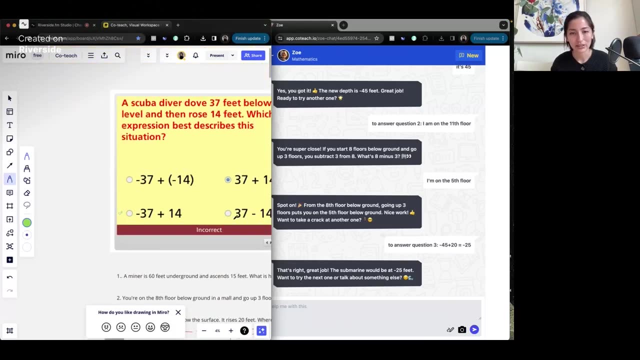 Yes, Okay, I got it right. A hiker starts a hundred feet below, below the top of the hill, And climbs up 22 feet. How far below the top are they? So that's a hundred minus 22,, 78.. 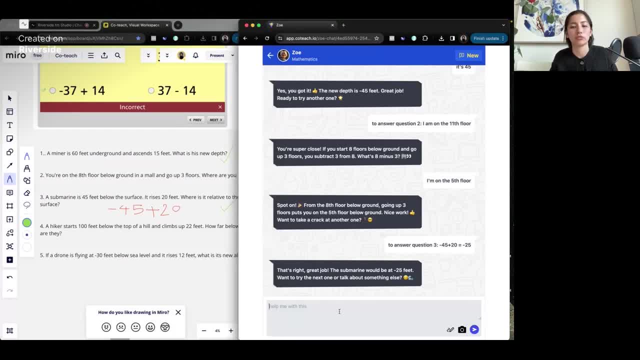 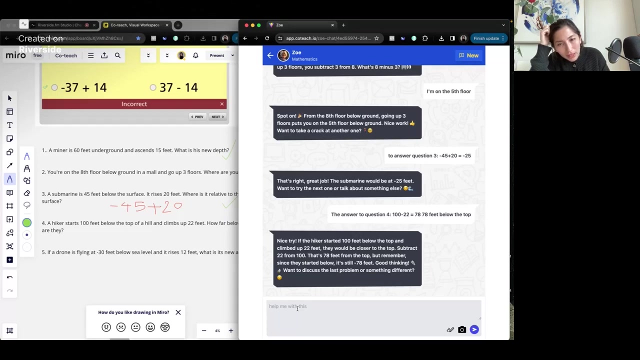 A hundred feet below and climbs up 22.. So the answer to question four, 100 minus 22, equals 78 feet below the top. They would be closer to the top Subtract 22 from 37.. Oh, it's negative 78.. 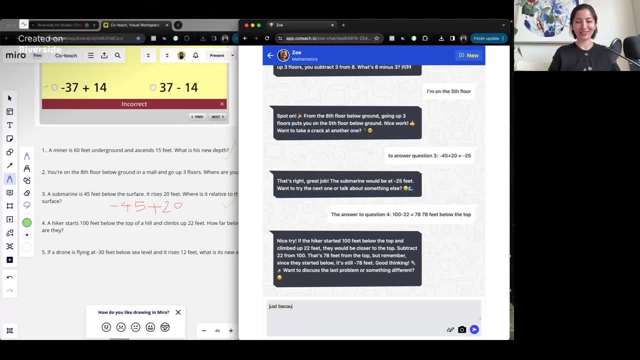 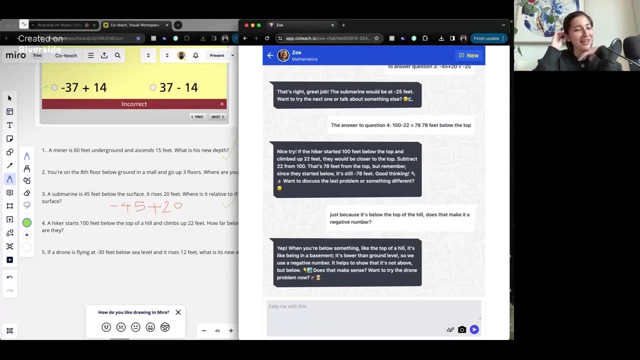 Yes, But just because it's below the top of the hill, does that make it a negative number? When you're below something like the top of the hill, it's like being in a basement. I don't know Explain it again. 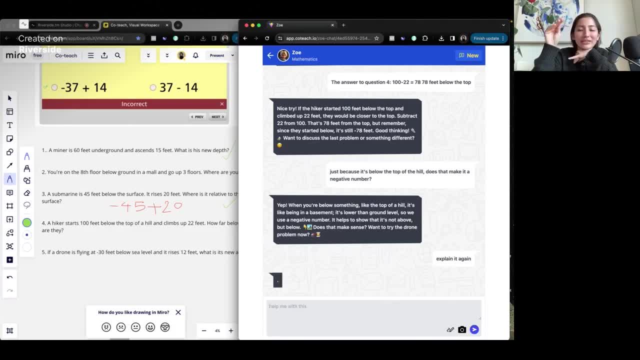 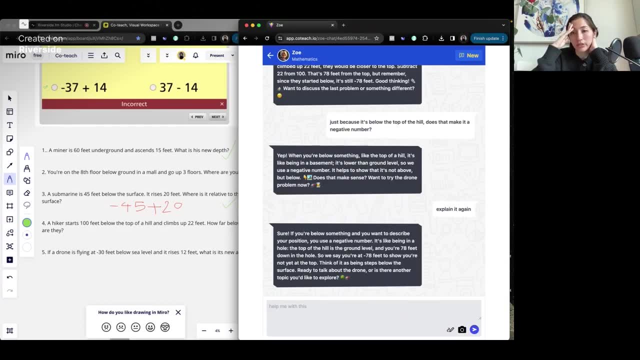 I just don't get why, just because you're at the bottom of a hill, it means it's a negative number. If you're below something and you want to describe your position, you use a negative number. It's like being in a hole. 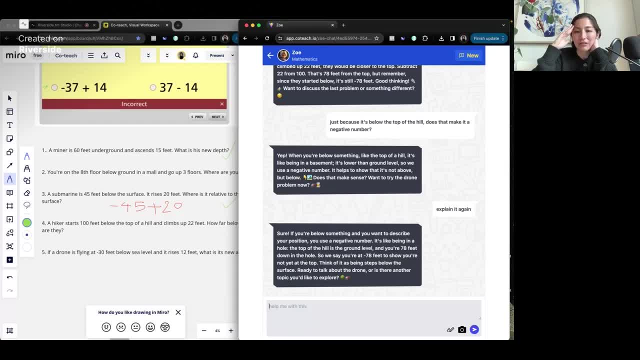 The top of the hill is the ground level and you're 78 feet down the hole. So we say you're at negative 78 feet to show you're not yet at the top. Think of it as being steps below the surface, Okay. 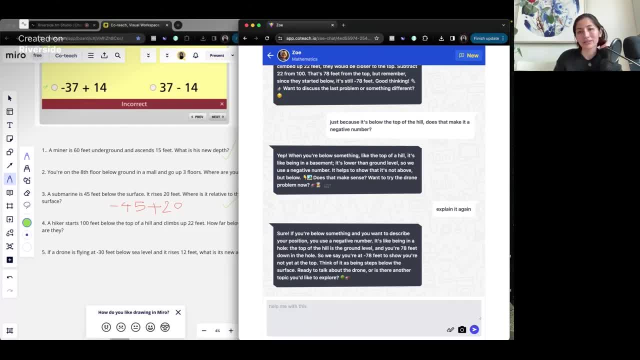 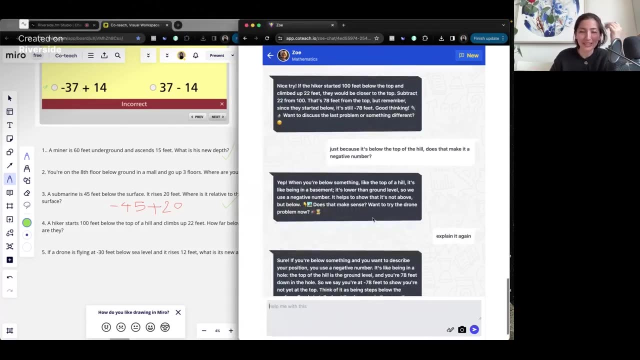 I mean, ideally Zoe should be asking if that makes sense. Oh, but she already did that. Gosh, we really need a way to make this like something to like help prompt alternative explanations. Okay, fine, Negative 78.. I got that one wrong. 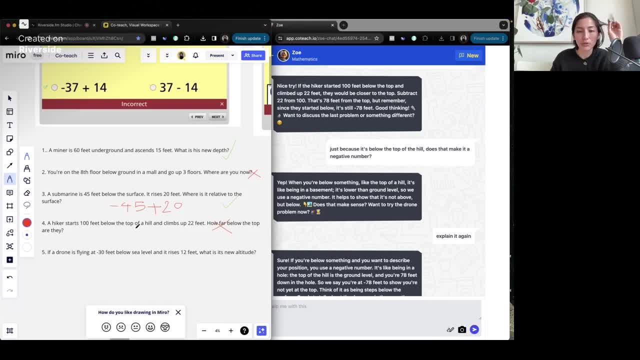 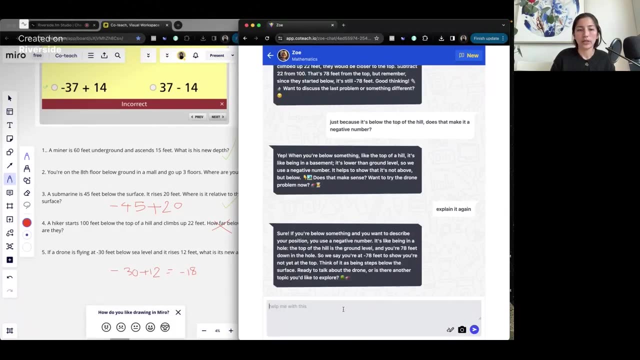 If a drone is flying at negative 30 feet below sea level and it rises 12 feet, when is its new altitude? Okay, so that's negative 30 plus 12. Which equals negative 18.. Okay, the answer is negative 18.. 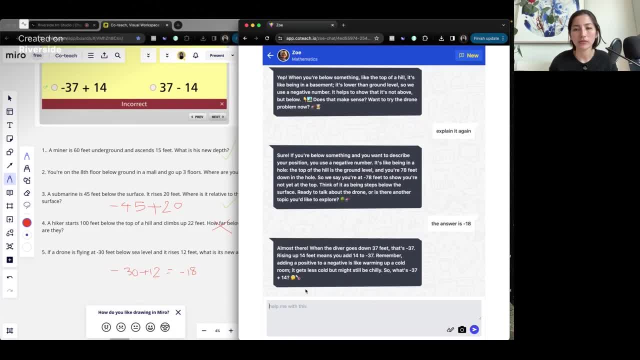 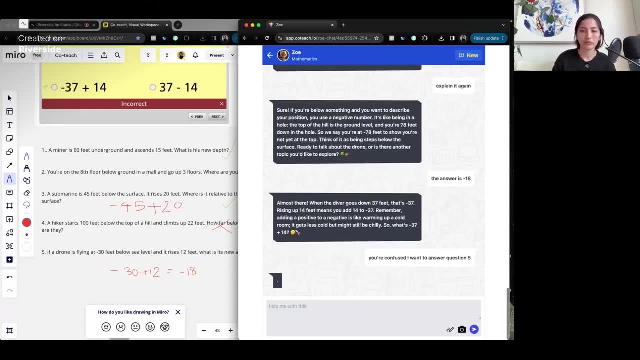 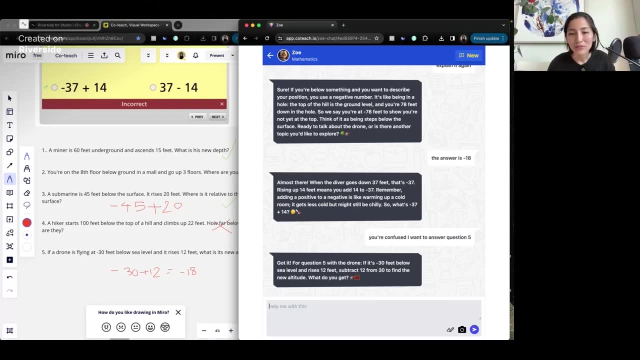 Oh, no, no, no, no, no. You're getting confused. now, Okay, You're confused. I want to answer question five. What if we had kids? just tell Zoe that they're confused, that she's confused. If it's 30 feet below sea level, subtract 12 to find a new altitude.